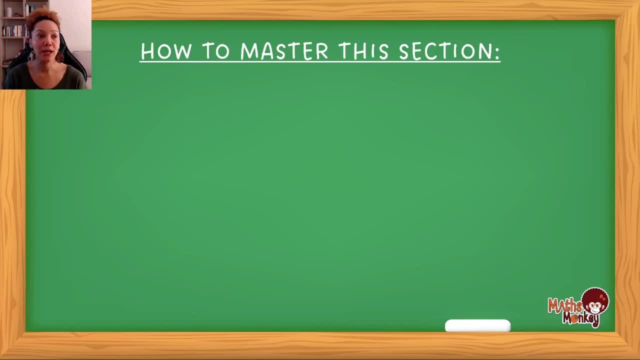 to answer this specific question paper that I'm going to work through in this video, because you're never going to see this question again in the final exam paper. Okay, but what I'm using these questions as is to guide you and to show you how you need to approach these types of questions. Okay, 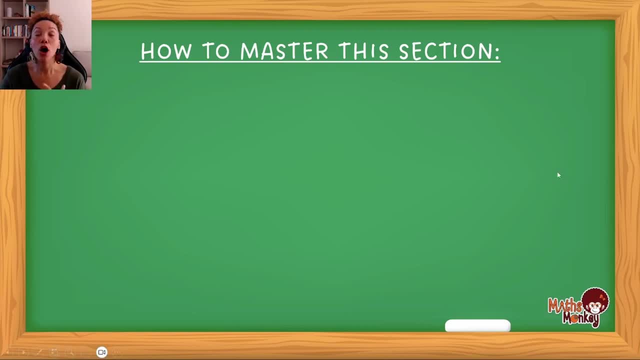 so, when dealing with these topics, there's a couple of concepts that you have to be clear and make sure that you understand. First of all, you need to understand that profit will always be your income minus your expenses, And if your income is more than your expenses, then you'll have a profit, But if your income 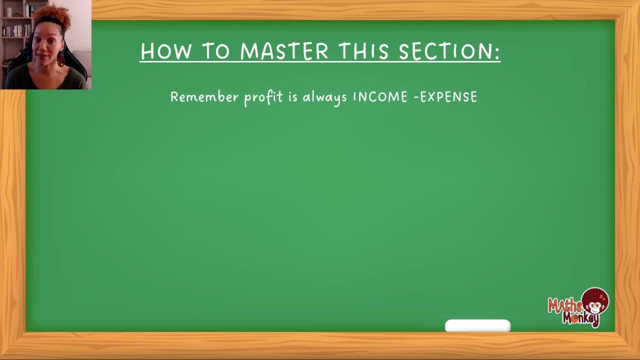 if your expense is more than your income, then you end up actually having a loss. Okay, so that's just the profit, understanding what profit and loss is. then we have: expense is what, what it will cost you. So money that's leaving your pocket, and income is money that's coming in. Okay, so these are just 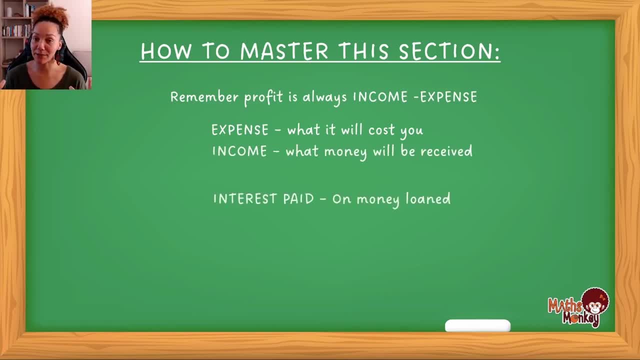 simple terms, That if you don't understand this, then whatever I cover is going to be a problem. Okay, then we have interest, right, so interest paid. So interest that me as a person and individual has to pay would be: if I loan money, So if I take out a bond or I have a car loan, that means that I have, I get that money. 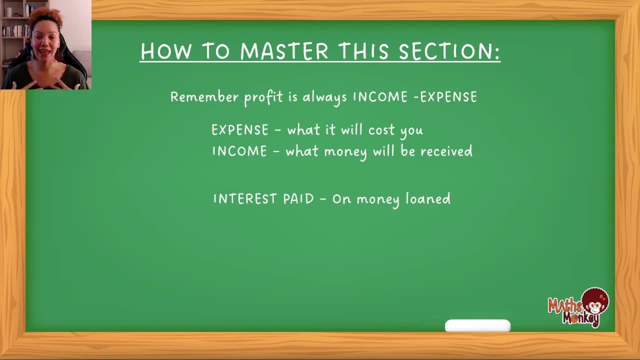 I'm borrowing that money So I have to pay back extra. So the extra that I pay back is the interest right. Also, I receive interest If I invest my money, so if I put my money in a bank or I put my money in a financial institution. 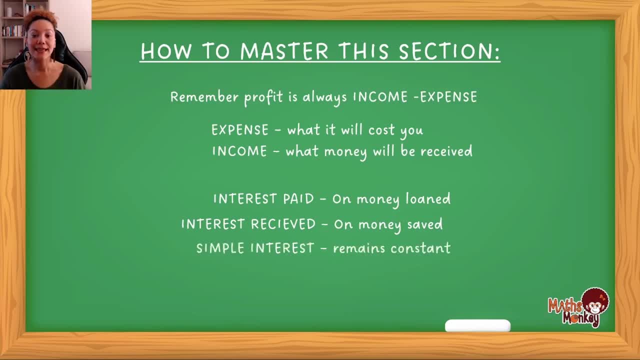 they then will give me my money back with interest. Right, Then we have two types of interest. By now you should have full understanding on simple interest. that is when they calculate your interest from the beginning and you just earn the same interest along, let's say every year or whatever the 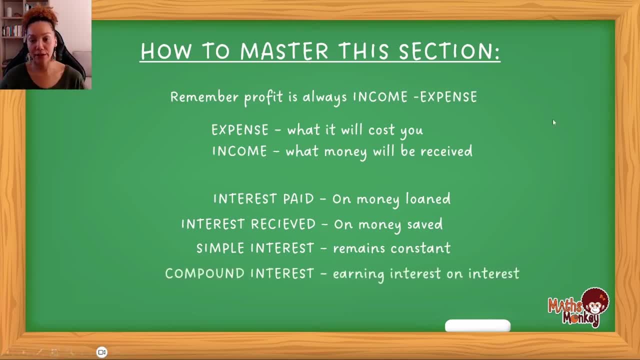 time period is that you've agreed with a bank. Compound interest, however, is earning interest on interest, So that means that you are not going to be like simple interest, be earning the same interest every year you're actually going to every year for compound interest. be earning interest on the interest that you even earned in the. 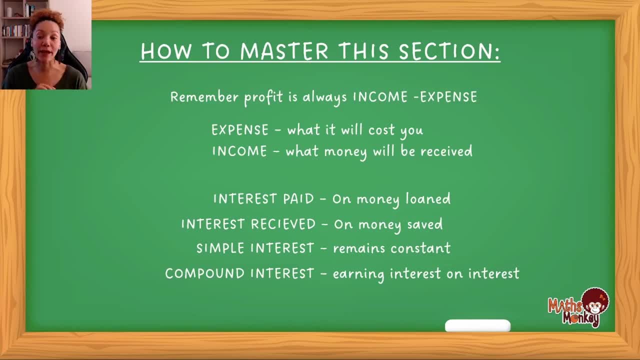 previous year and on the original value. Now I've made a video on each of these, So please feel free to have a look at my finance playlist on my channel for grade 12 mathlet, And there you will find a video on each of these. 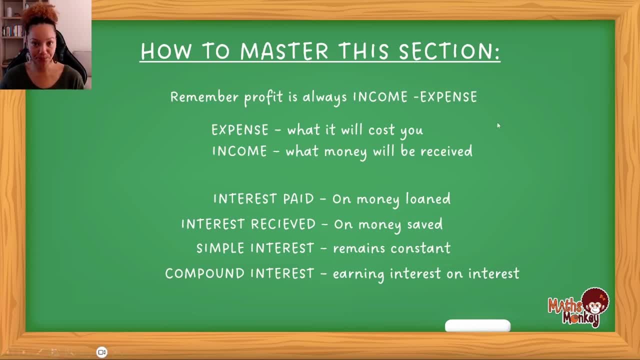 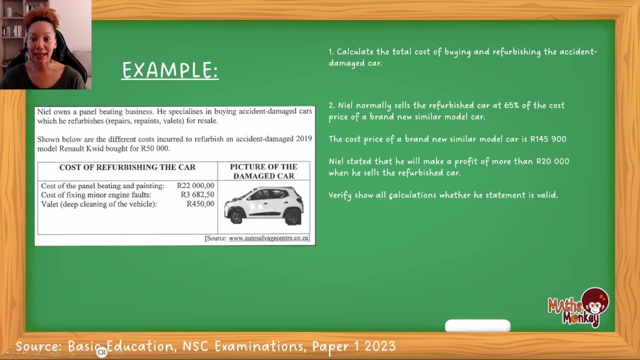 And you can delve into them individually if you so wish. Okay, so now let's actually look at a question. So what I've done is I've cut out the scenario from the question And I've typed out these questions. So these are actually the questions from the question paper. are for the NSE exams. Okay so. 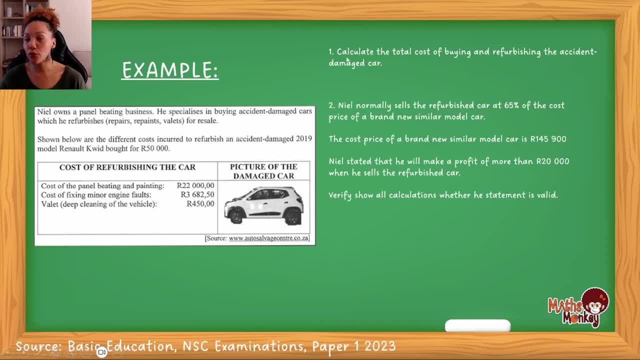 let me take you through this. So when you get a question like this, before you even read questions, you have to make sure you read all the information that's given to you. you understand all the information that's given to you before you actually attempt the questions. 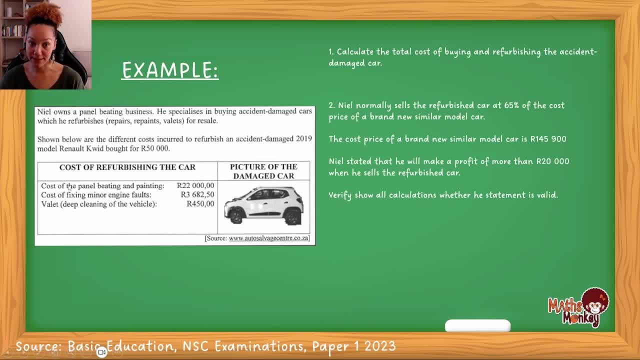 So let's work through this. Neil owns a panel beating business. He specializes in buying accident damage cars which he then refurbishes, repairs, repaints, valets for the sale. Shown below are the different costs incurred to refurbish an. 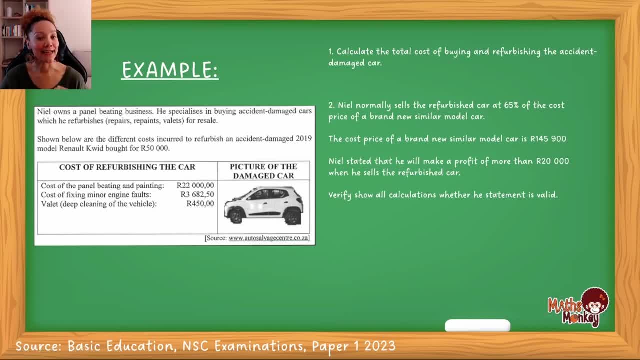 accident damage. 2019 model Reynold Quidd bought for 50,000 Rand Cost of refurbishing the car. So here they're: give you the three costs of what it would cost you to fix the car and then the actual picture of the car. Fine, I've read all. 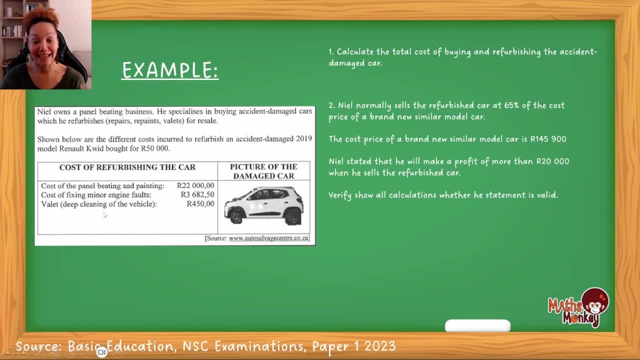 the information that's given. I make sure I understand all the information. Now I'm ready to actually read the question. So the first question asks: calculate the total cost of buying and refurbishing the accident damage car? So yeah, they say that. 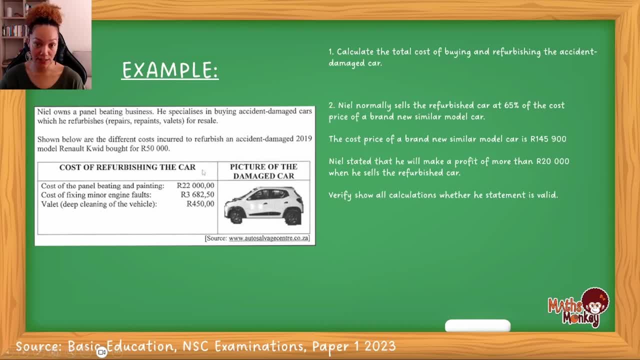 the car was bought for 50,000 Rand. And then they give you these three totals are to refurbish. So we will say 50,000 plus the 22,000. Plus the 368 to 50 plus the 450. And in total it would cost us- save the cost, Neil- 76,132.. And 50 cents, Okay. so that is. 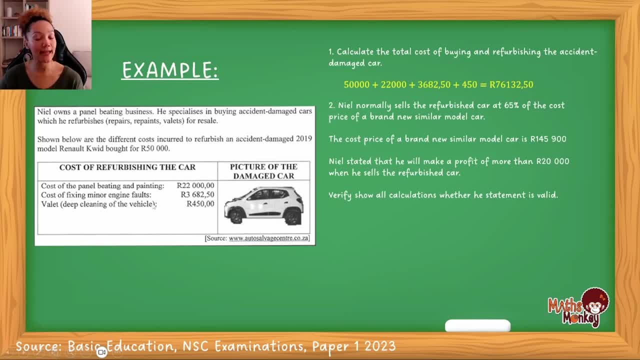 simple. That is just making sure you read all the information correctly And that you actually just extracted all the information to answer the questions. That's fine. Let's read the second question. The second question says Neil normally sells the refurbished car at 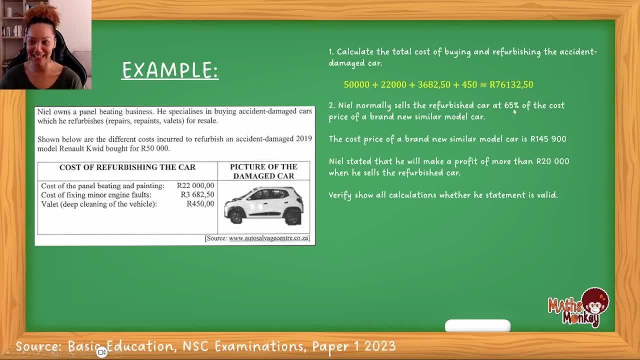 65,000.. At 65% of the cost price of a brand new similar model car. The cost price of a brand new similar model car is 145 900.. Neil stated that he will make a profit of more than 20,000 Rand when he sells the refurbished car. Verify show all calculations. 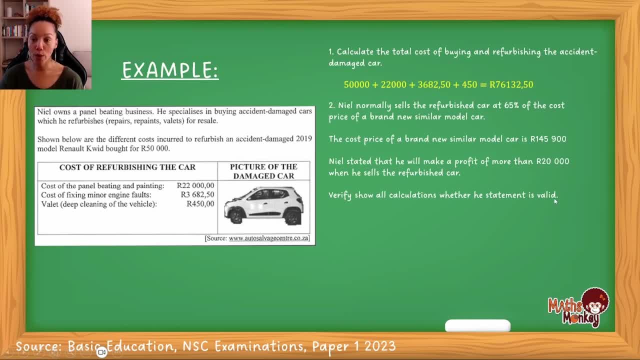 whether his statement is valid. Okay, so what they say here is he sells the score right for 145 900.. Sorry, though, he sells it at 65% of what a new car for that same model would cost, And the new car would be 145 900. 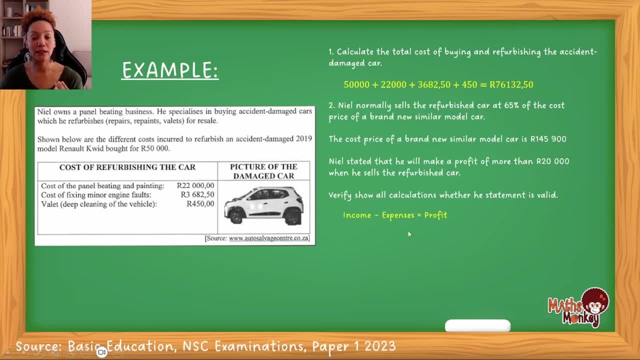 So the way we would approach this is: we would note that profit is equal to income minus expenses, right? so his income for this specific car would then be what he's actually going to sell the car or plan to sell the car for. so that's 65 percent of 145 900 and it will give. 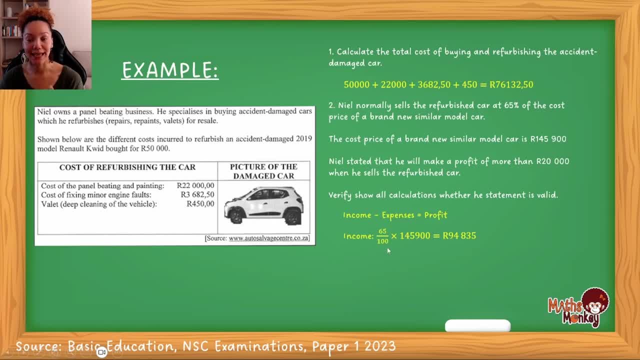 you nine, four, eight, three, five, so again money that's coming to him would be the money that he's actually going to be selling the car for. so they tell us that he sells the car at 65 percent of the cost of a new car, which is then 65 percent of the 145 900, which gives us the nine, four, eight. 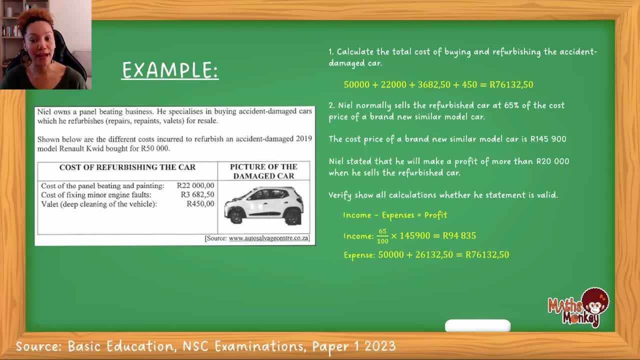 three, five. that is our income now. if we look at our expenses right, this is again this value over here, which is the 7613250. that's what it's going to cost him. it's going to cost him 50 000 rand to actually buy the car for him. so that's what he's going to be selling the car for. so that's. 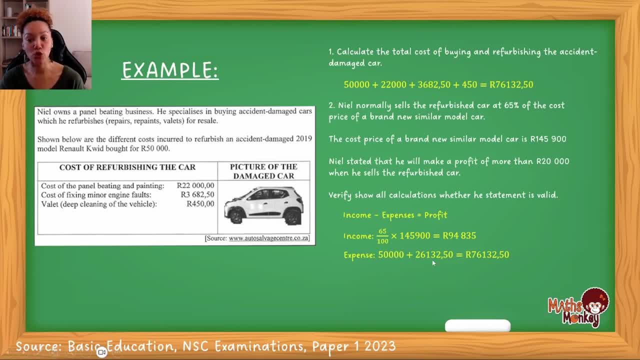 buy this car that was in the accident and then 26 132 rand and 50 cents to fix it. so all this money has left his pocket and he then has 76 000. he has paid 76 132 and 50 cents now to find the. 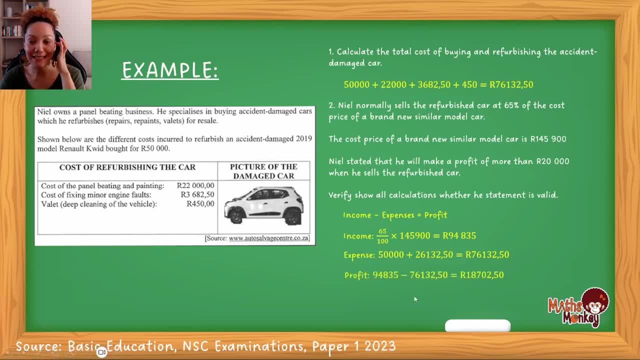 profit. we then say income minus expense and i end up having 18 702 and 50 cents, which is how much he would make, you know, on this car. okay, now the question says that neil stated he would make a profit of more than 20 000. 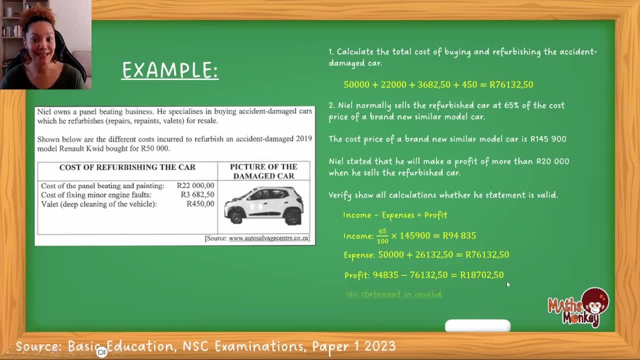 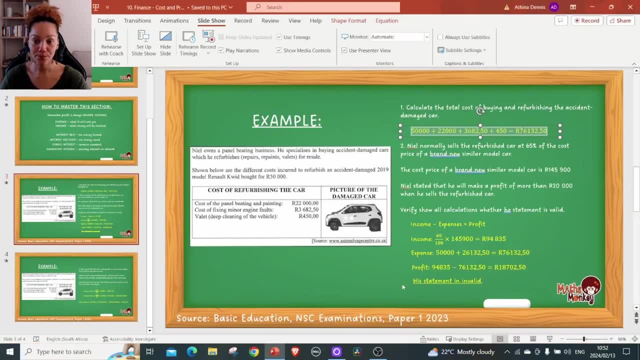 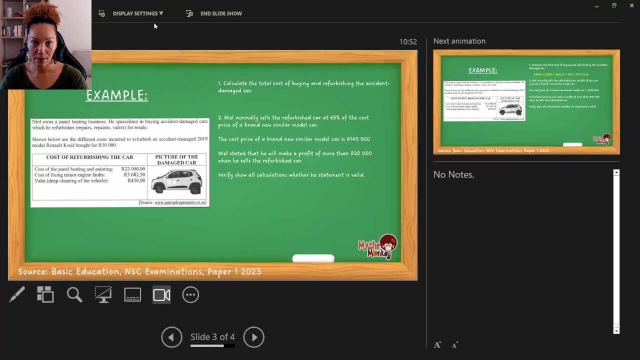 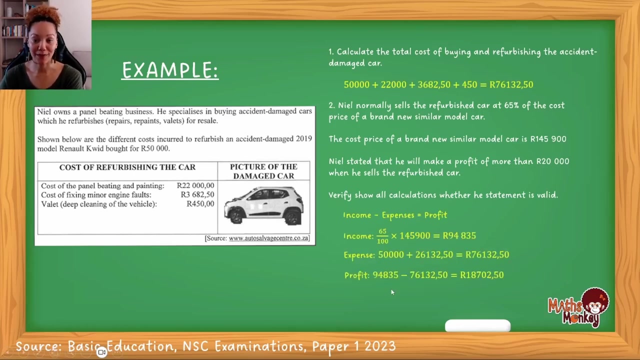 but that is not the case, based on the information given to us. so therefore, we have to actually conclude the question by saying this statement is invalid. conclude the question by saying his statement is invalid. okay, so again, do you take note here that you wouldn't know how to answer these questions if 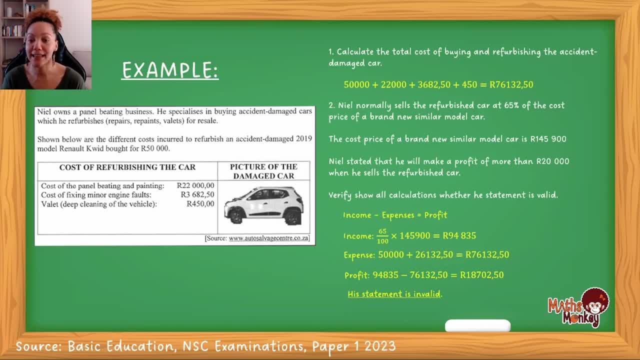 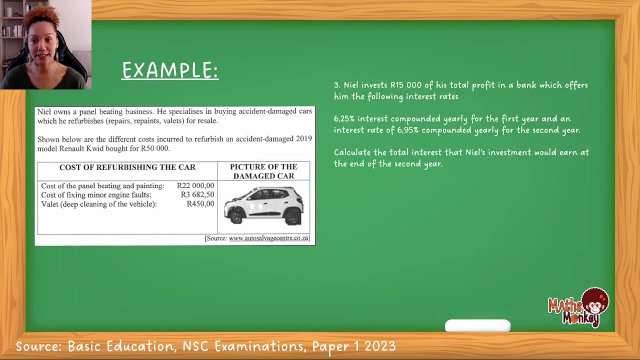 you didn't understand the concepts of profit and understanding that you wouldn't know how to answer them all. so we have bases here. so here we have the whole process of profit analysis. you've got different versions for 4, 11, Shop לע 10, 11. 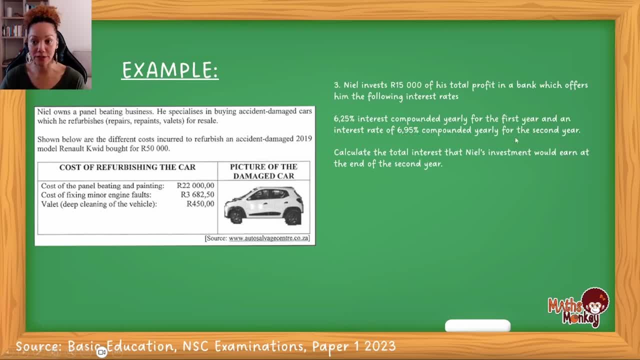 12, 13, 14, 16, 17, 18, 13, 17, 18, 17, 18, 20. the total interest that neil's investment would earn at the end of the second year. okay, so he invests 15 000 for the first year. this is the interest. he gets 6.25 for the second year. 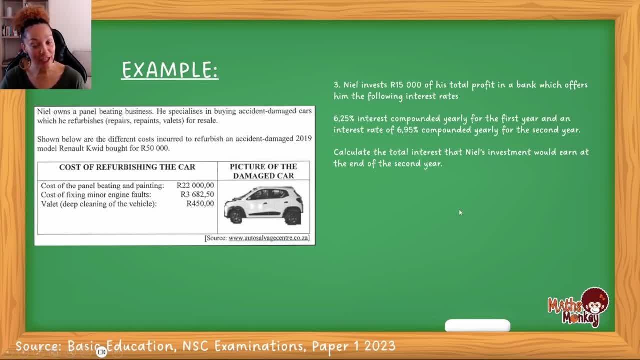 this is the interest he gets, which is 6.95. so to answer this question, we're going to do it as follows for the first year, right, his interest, which was 6.5 time over 100 times what he invested. so 937 and 50 cents is what he makes in the first year. okay, now the total amount of money that he. 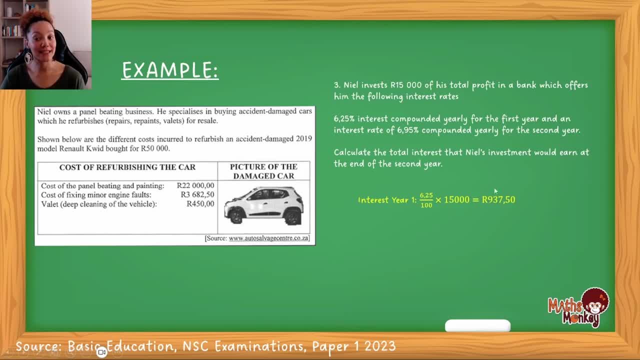 has he has in the account is the fifteen thousand plus this nine, three, seven and fifty. so when we calculate the interest for the second year now, we're gonna calculate the six point nine, five, five times both of these values because, remember we said compound interest is interest earned on.